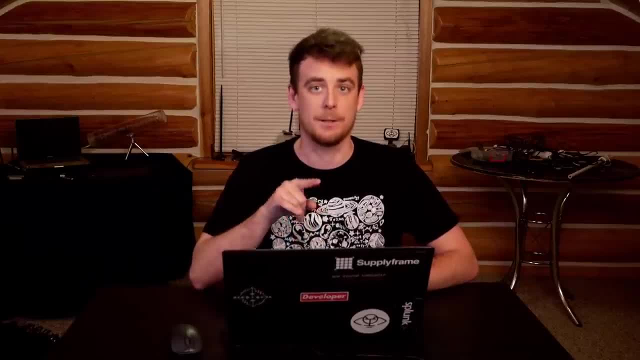 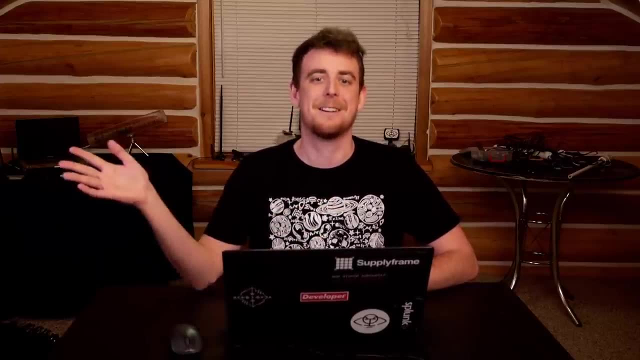 And also you're going to need to be running Linux. I'm using Ubuntu, You can also be using Kali or, I think, any other Linux distribution would work. So, without further ado, let's get started. So, in order to test our SQL injection attack, we're going to need to run some tests. 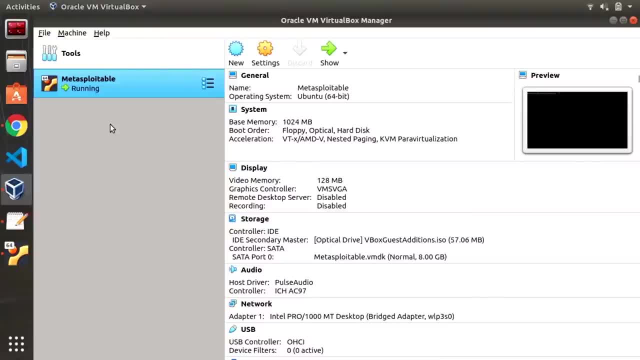 We're going to be using Metasploitable. Metasploitable is an operating system that was designed to be hacked, And one of the services it offers is a server that is vulnerable to SQL injection, So let's go to our. I'm running Metasploitable in VirtualBox. Let's go to Metasploitable. 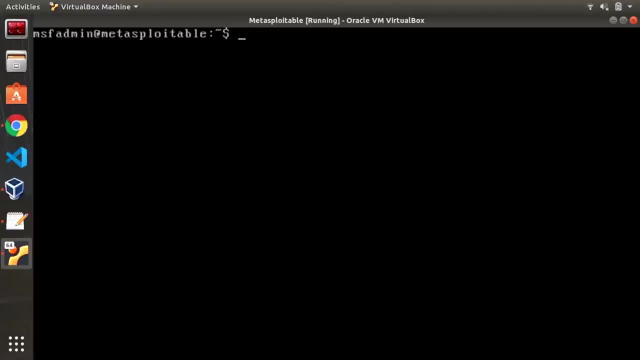 I've logged in as msfadmin, which is the default account for Metasploitable, And I want to find the IP address of our server of this machine. So I'm just going to type in ifconfig And I'm going to look for the inet address. So I'm going to do pipe gret, inet. 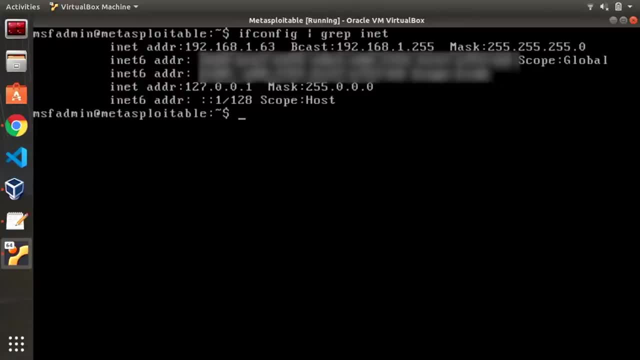 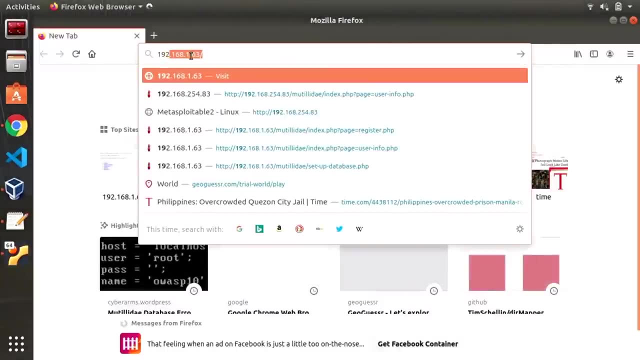 And I want this IP address at the top, which is 192.168.1.63.. So let's go to a Firefox browser And then let's go to that IP address. All right, so you can see right here, this is the splash page for the Metasploitable server. 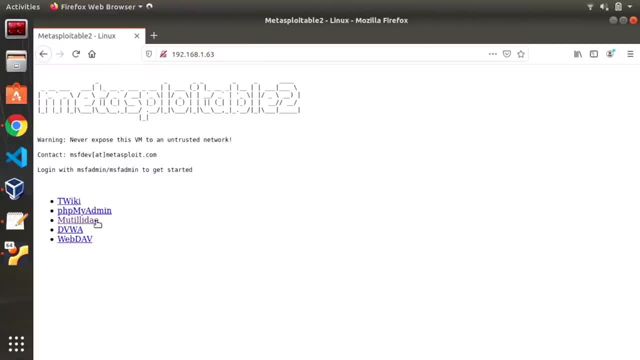 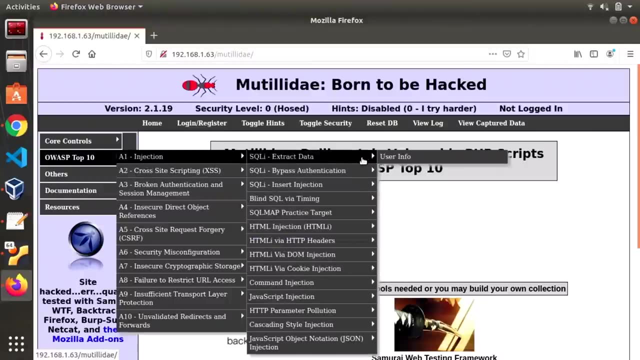 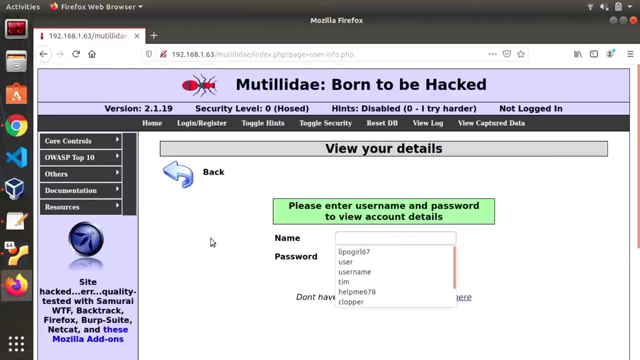 We're interested in this particular site, Mutiliday, And on it in the OWASP 10 section there's injection And SQL extract data user info right here. So this is what you would find on many websites. It's a login portal. 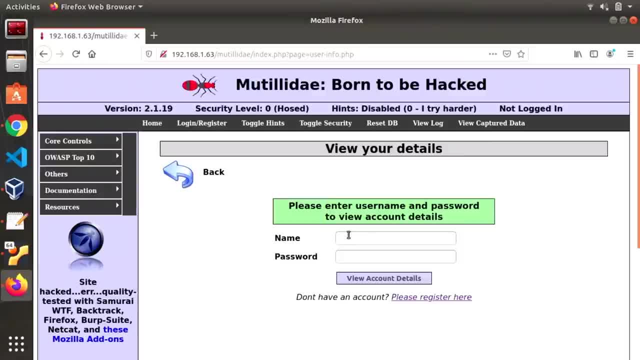 And this one is vulnerable to SQL injection. So this is kind of our test bed. So once we're here we don't really need to do anything. Mutiliday already has a host of other accounts that have already been created that are in the database for this server. 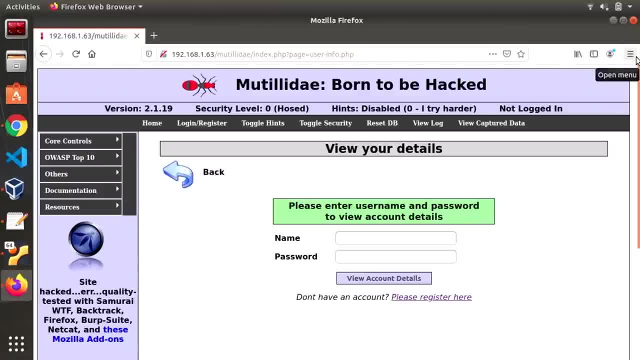 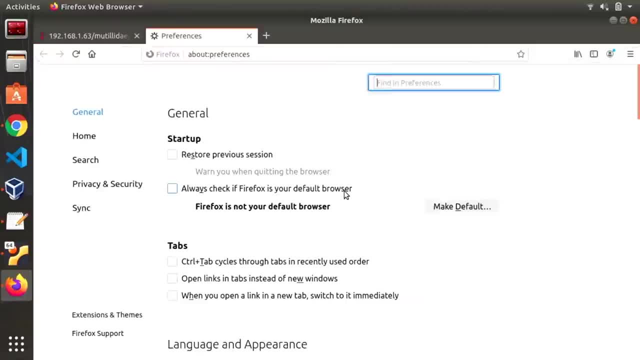 And all we need to do is attack it with BurpSweep. So before we load BurpSweep first, what we want to do is we want to go into our Firefox settings. We're going to go down to the bottom and we're going to change the network settings. 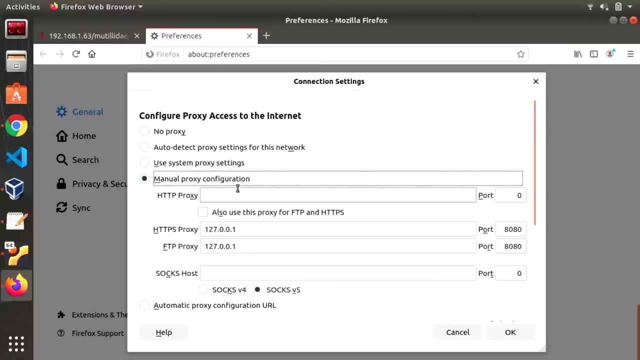 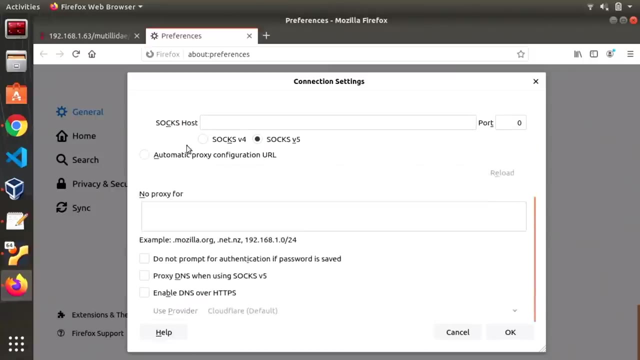 Now we're going to switch to manual proxy configuration And for this video we're going to do 127.0.1.. I'm going to go on port 8080.. Make sure this box is checked And no other thing is checked. 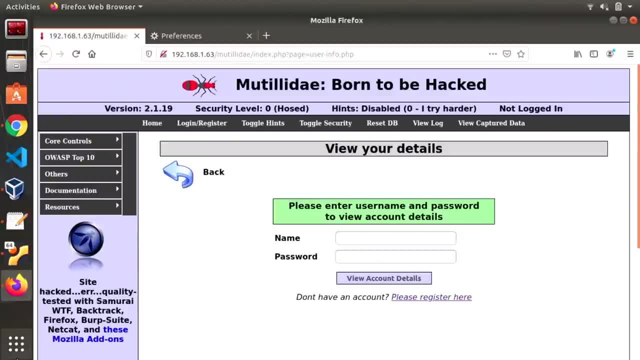 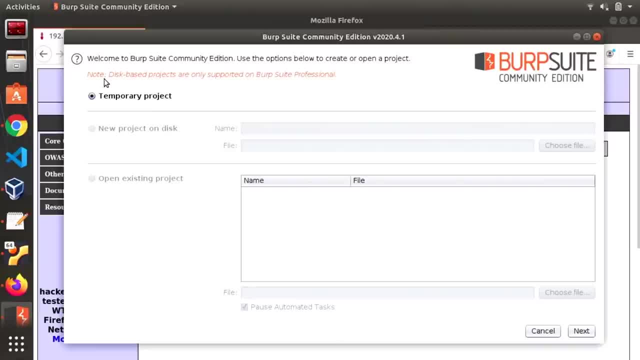 Let's go and press OK. Alright. so now we're running through a proxy And let's start BurpSweep. Okay, so BurpSweep. this is the Community Edition. There's a lot of features that are disabled. 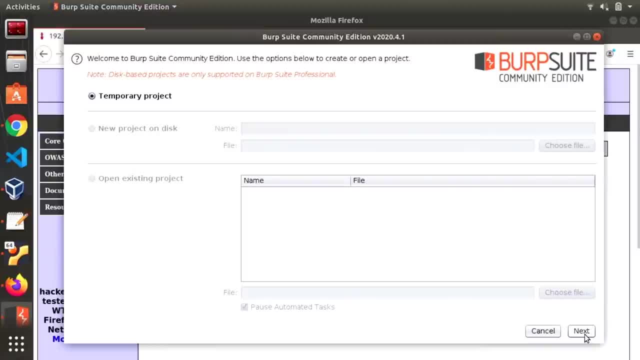 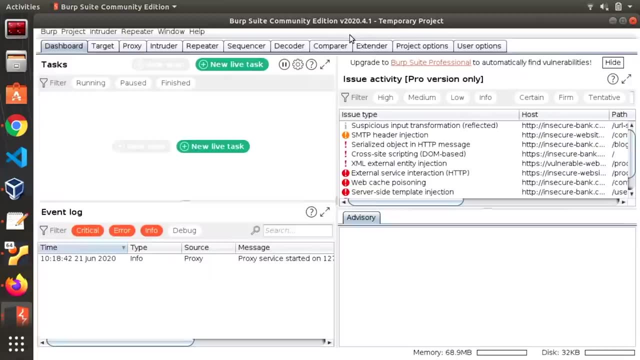 But thankfully SQL injection is still something that we can do with the Community Edition. Let's start a temporary project, Use the Burp defaults And start Alright. so there's a lot going on right here. Don't need to pay attention to any of this. 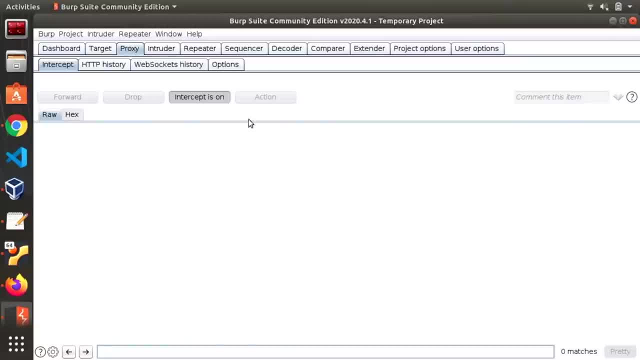 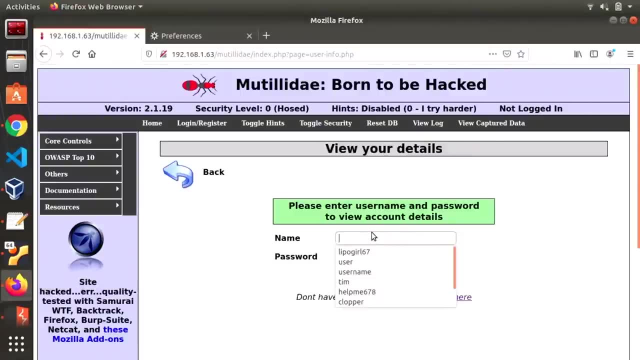 The first thing we need to do is we need to go to proxy And we see intercept is on To test this. let's go back to utility in Firefox And let's type in username. I'm just going to go with password. 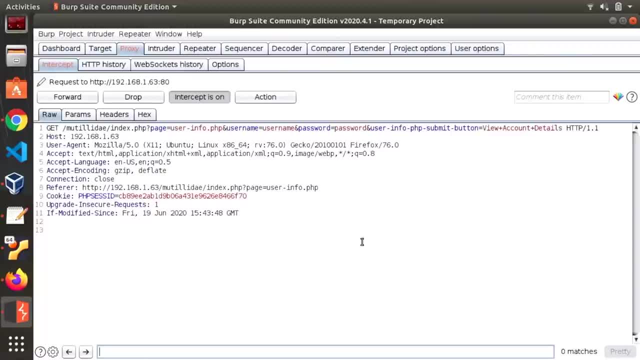 Press enter Alright. and now we can see BurpSweep has captured all of the raw HTTP that's gone through here. So once we have this, the next thing we need to do is we need to send this to the intruder. 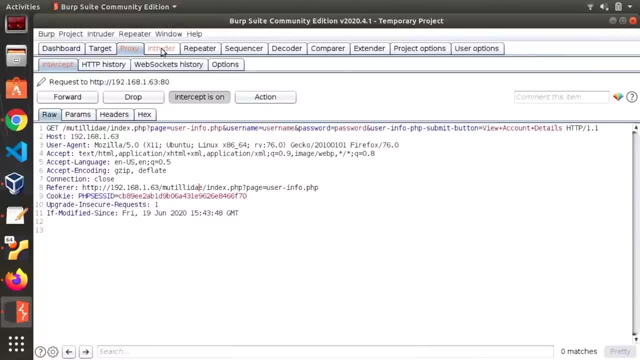 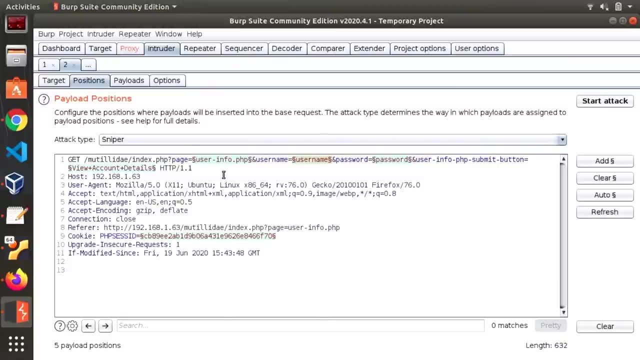 What that lets us do, if we go over to the intruder tab, is we can go to the positions And we can see the same information was sent here. This lets us edit the HTTP request. So let's first we need to clear everything. 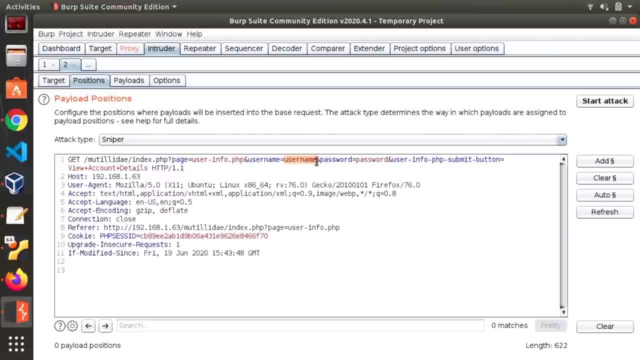 And what we're particularly interested in is we're interested in injecting SQL code in the username field. So we're going to highlight the after pressing clear, we're going to highlight what we entered in as the username. In this case, I kind of confusingly just entered username. 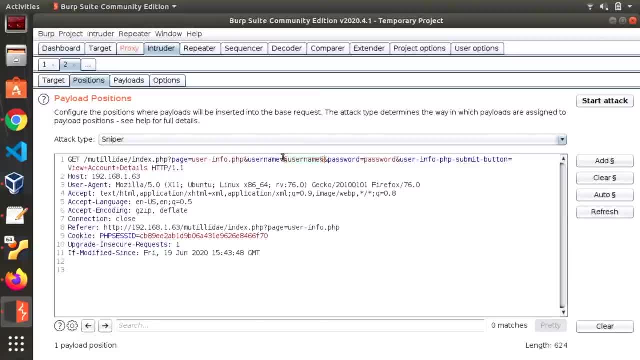 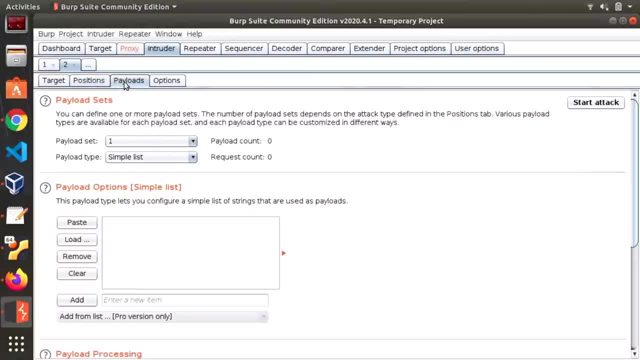 And we'll see that And we're going to click the add button with that highlighted. So that's where it's going to inject our SQL code. Alright, so we're actually almost done. The only thing we need to do now, since we aren't writing any of our own SQL code. 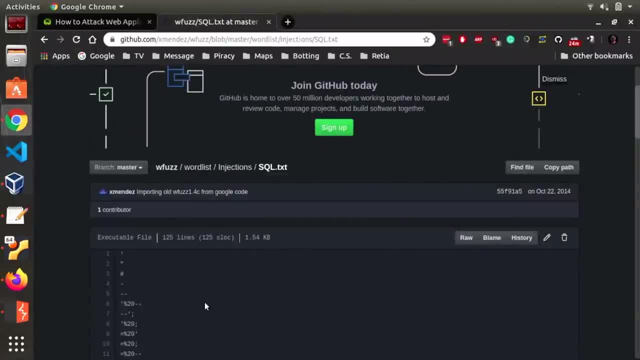 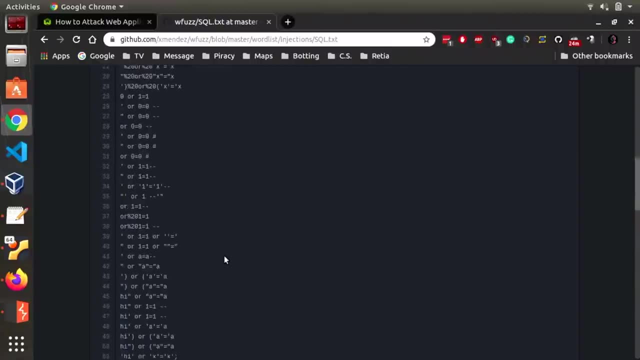 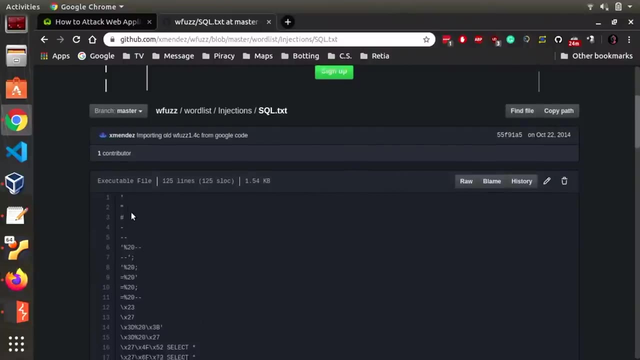 we're using a list of basically SQL injection words or strings that someone else has created. I found this one on GitHub And I also believe this is the default one that comes with Kali Linux. I'm using Ubuntu. Obviously, it's not designed for attacking, so it doesn't have that word list included. 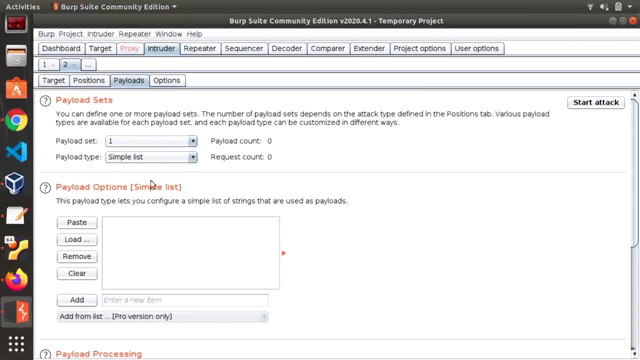 But I just downloaded this, So go back to BurpSweep. I'm going to load that list right here. Open it And you can see all of the strings are right here, And once we have all of those loaded, we just have to start the attack. 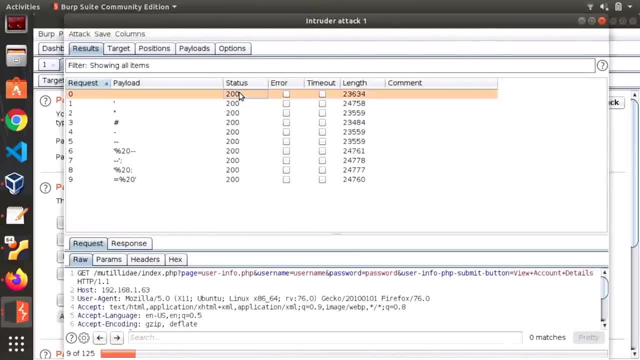 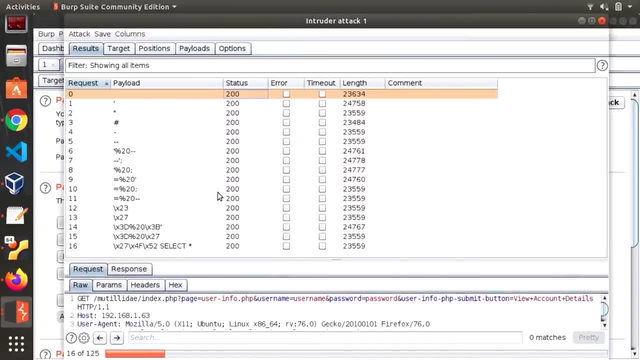 As you can see, we're getting, with each string we're getting the status 200, which is good. That means okay, That means we successfully were able to fulfill the request. And when we look at all of these strings that we've tried, we look at their response. 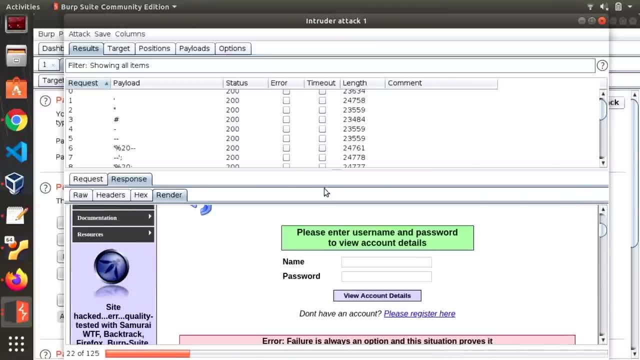 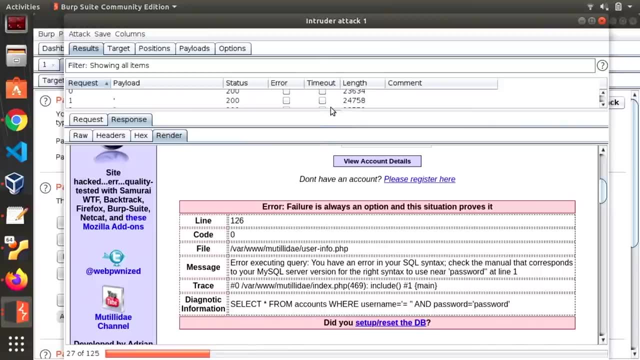 and we can go to the render tab and see basically what happened when we tried to enter in that one, For instance this one- there's a failure. It basically says that the SQL syntax wasn't correct. But if we look at a different one, I know number 39 works because I've tested this- 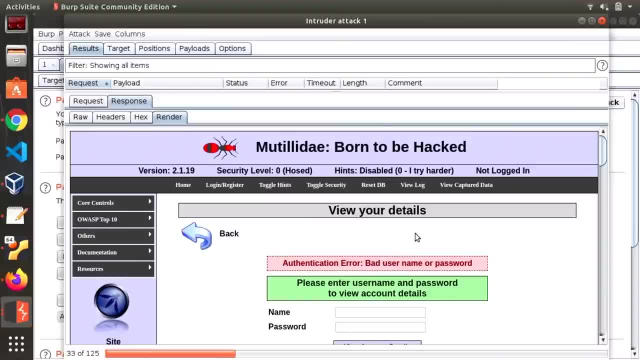 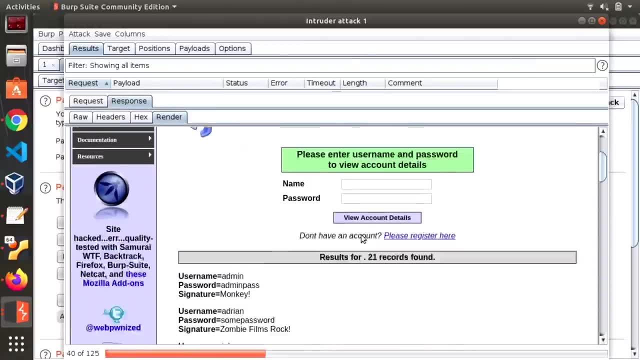 But some of these work and some of these don't work. That's why we have a full list of them. This one has an authentication error, All right, And if we go to number 39, we should. yeah, there we go. 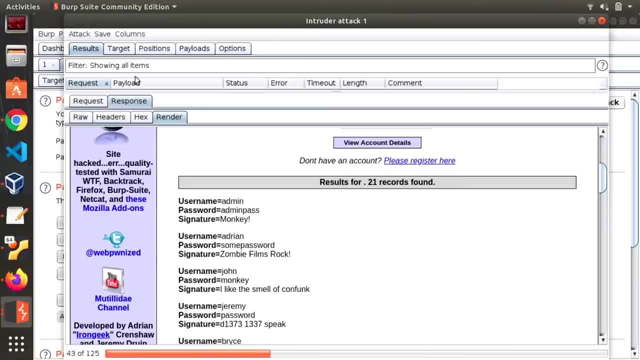 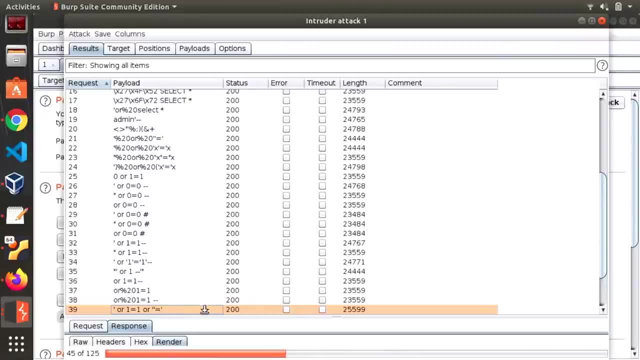 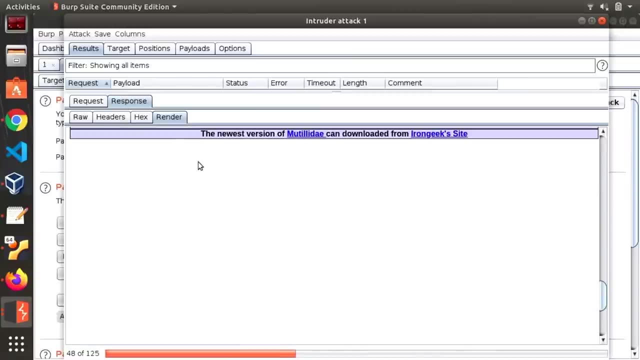 So we can see that this particular SQL string- what was it exactly? It was end quote, or one equals one, or double quote equals single quote. So yeah, that particular SQL string. we were able to essentially display everything in the database, So you can see all of these different usernames and passwords and their signatures. 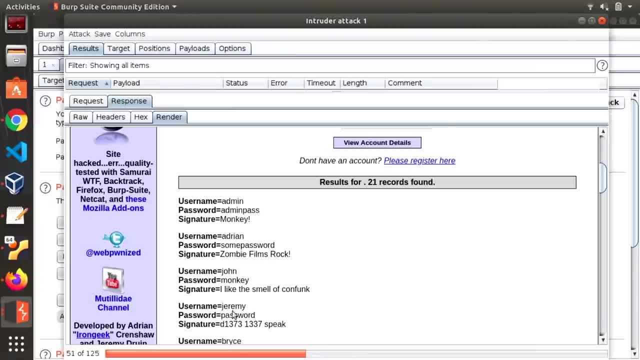 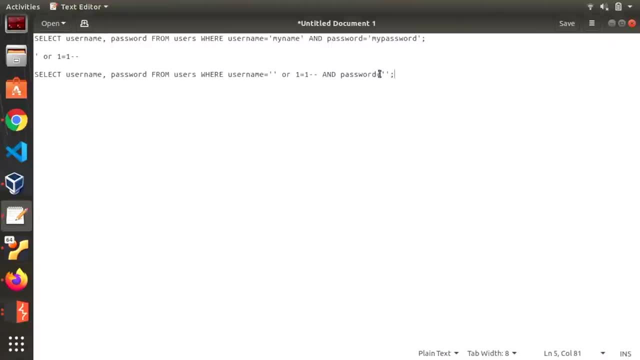 The entire database of the login credentials is now ours, And the reason this works is because of SQL itself. So I typed a little example right here. So when we're entering a username and password into those fields on the web page, it makes a SQL query. that's usually structured something like this: 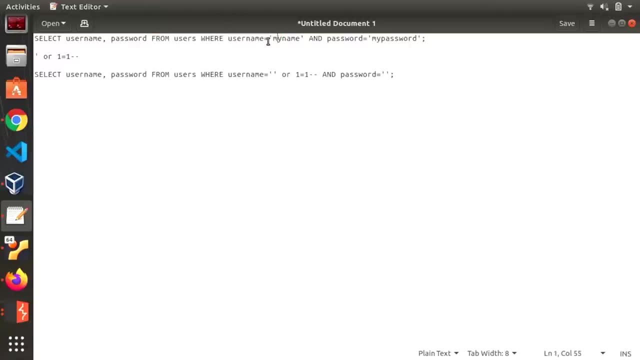 Select username password from users where username equals my name, which is the username that you typed in, and password equals password- My password, which is the password you typed in. Now, when we put something in the username field like end quote or one equals one dash dash. 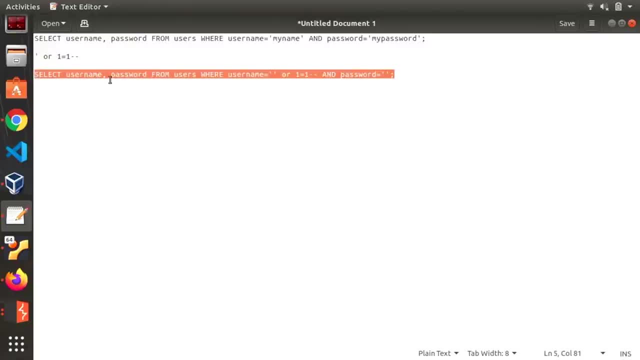 for instance, what we're doing is, when the SQL query is run, where it asks where username equals, it basically says: blank right here, or one equals one, which always evaluates to true, And then these double hyphens will negate anything after them. 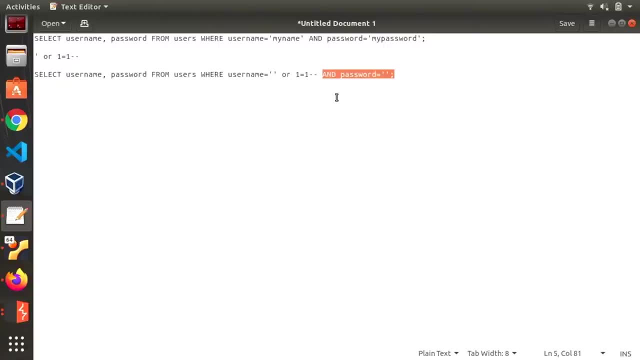 So the end password is irrelevant. So basically, since one equals, one evaluates to true, it's going to select every single entry in the database and display it for us. So yeah, that's just a little insight into what's actually going on. 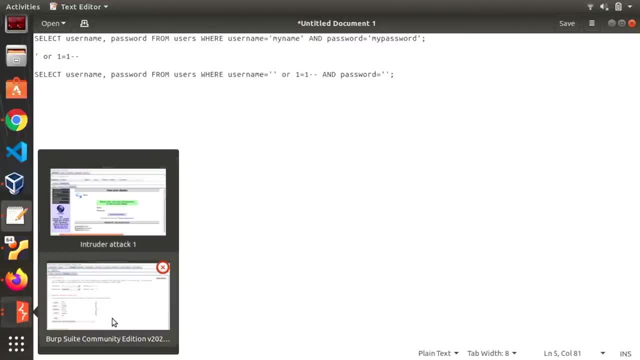 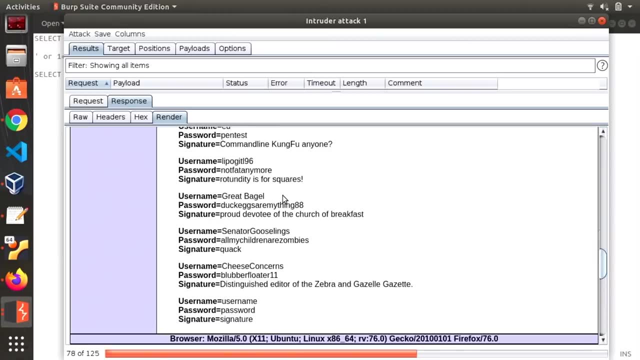 But you don't even need to know that. with burp sweep and with the SQL injection word list, We are able to totally see the entire database. So yeah, there you go. If you like this tutorial, be sure to check out our website, where we have hundreds of free articles and videos. 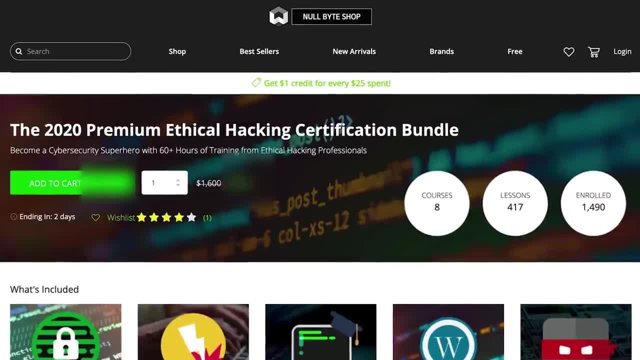 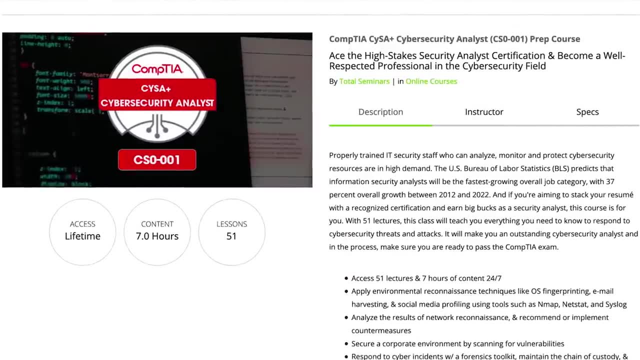 as well as premium paid content like the ethical hacking certification bundle, which features pen testing with OWASP, WordPress hacking and hardening and the CompTIA cybersecurity analyst prep course. Check out the link in the description below. All right guys, so that was pretty cool. 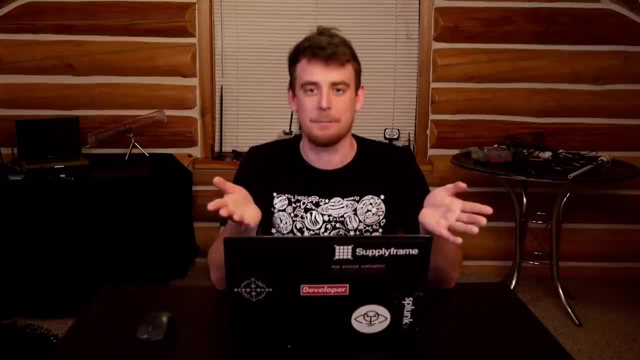 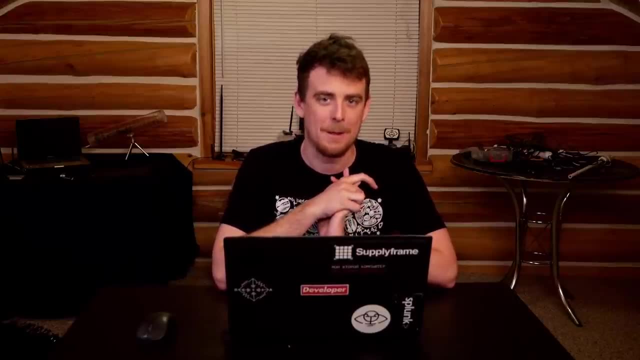 You saw, we were able to grab all of the credentials, all of the usernames and passwords from this web apps database, including some administration credentials, which is pretty cool. So if you want to go more in depth with this, you should probably learn some SQL yourself. 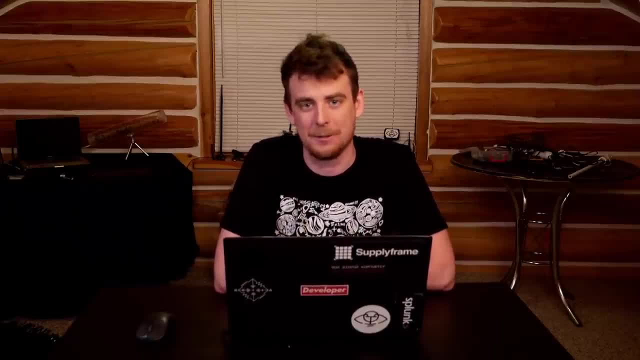 That way you can customize your tax. You can grab exactly what you want from the databases. Unfortunately, in the real world, any big company or large enterprise is not going to be vulnerable to this kind of attack, because there are specific coding practices that make databases basically impervious to SQL injection. 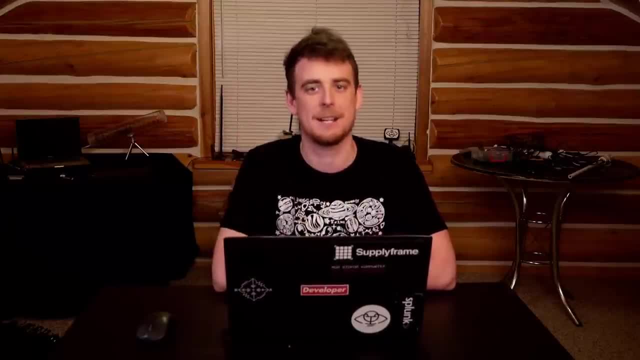 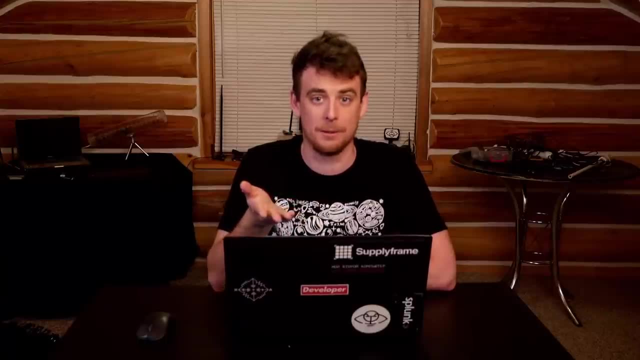 But there are plenty of small websites out there that you know. anyone these days can set up a web server with a database behind it And unless they're using those very specific coding practices, they will be vulnerable to SQL injection. So they are potential targets. 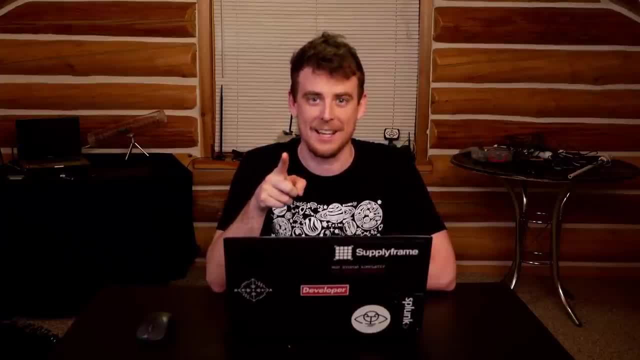 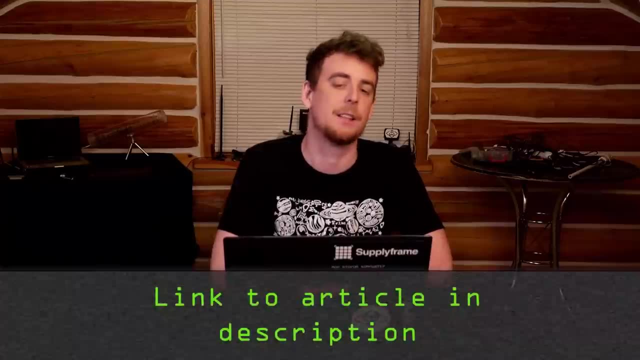 Although, of course, I do not condone attacking any websites that are not your own. If you want to learn more about SQL injection and about burp sweep, go ahead and check out the link to the article on this video's description, as well as the multiple other articles we have on Nullbyte about this topic. 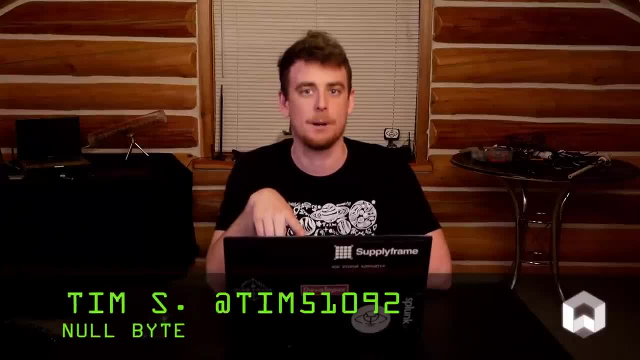 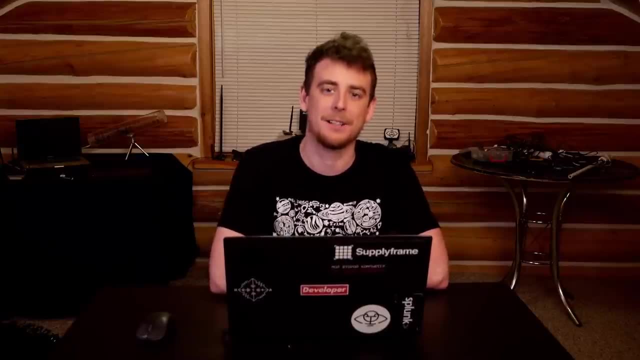 And if you have any suggestions for future videos, go ahead and hit me up on Twitter at Tim51092.. Don't forget to like, comment and subscribe to this video and have a good day. We'll see you next time, guys. Bye-bye.